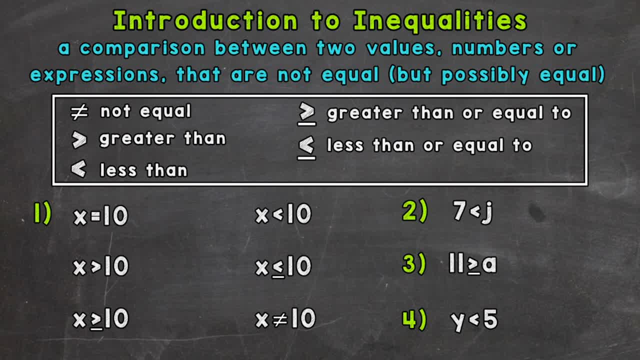 And we'll start with: x equals 10, which is not an inequality, It's an equation. So x equals 10.. This is an equation. Now, there's only one solution for this equation: x has to equal 10.. No other solutions will make this equation true. 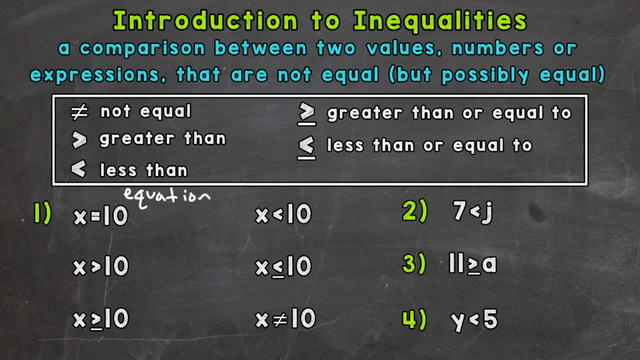 For example, if we were to plug in: x equals 9.. Well, let's put a 9 here. Would 9 equal 10? No, The only thing that x can equal is 10.. 10 equals 10.. 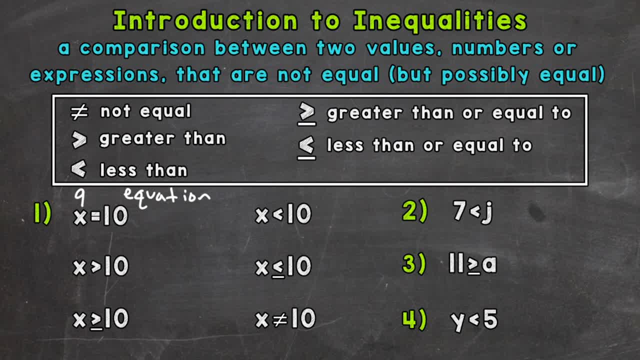 So I wanted to include an equation so we could compare this to the inequalities. Now for number two we have: x is greater than 10.. Now, remember, you always want the wider side, the open, wider side, of an inequality symbol facing the greater value. 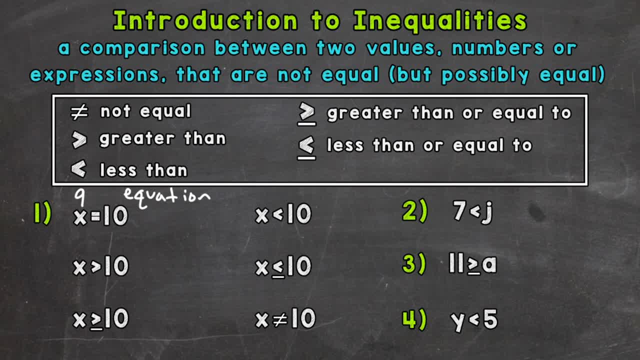 So x is greater than 10 here. So any number greater than 10 is greater than 10.. So any number greater than 10 is greater than 10.. So any number greater than 10 is greater than 10.. And 10 would be a solution for that inequality. 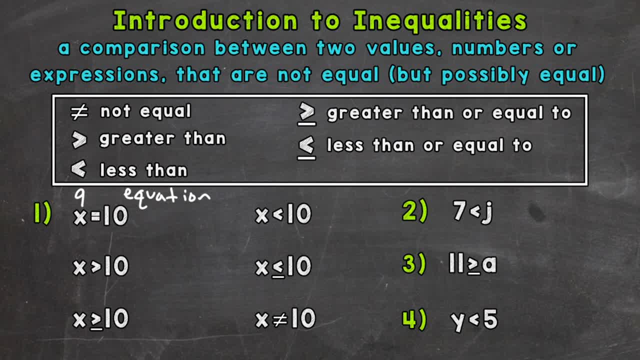 There's an infinite amount of correct solutions. So, for example, 11 would work, 50 would work or 150.. It doesn't matter. Anything greater than 10 would be a solution for x, for that inequality. Now, 10 would not be a solution because x has to be greater than 10.. 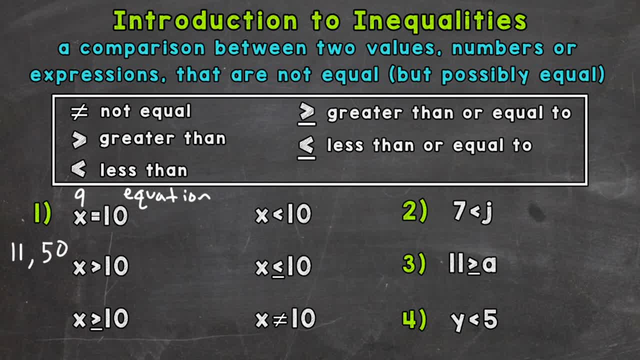 Is 10 greater than 10? No. Now the third inequality down right here is: X is greater than or equal to 10.. So all of those solutions we talked about, for X is greater than 10,, 11,, 50,, 150,. 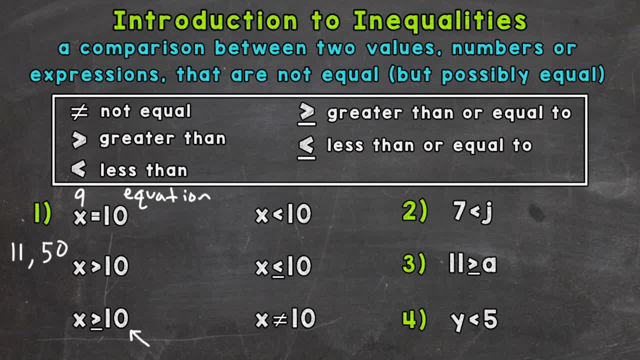 anything greater than 10 would be a correct solution, just like the one above, But this one, 10, is a correct solution as well. So 10 would work for this, because 10 is greater than or equal to 10.. So when we talked about the possibility of the values being equal, 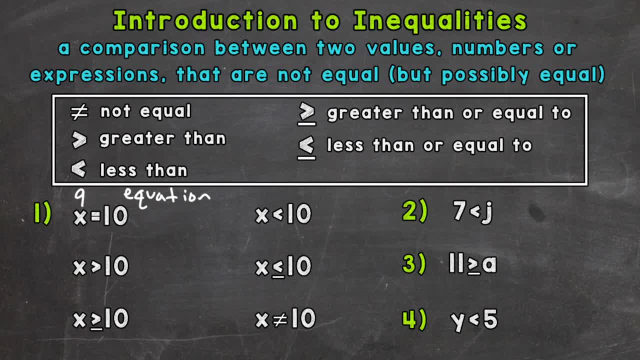 So I wanted to include an equation so we could compare this to the inequalities. Now for number two we have: x is greater than 10.. Now, remember, you always want the wider side, the open, wider side, of an inequality symbol facing the greater value. 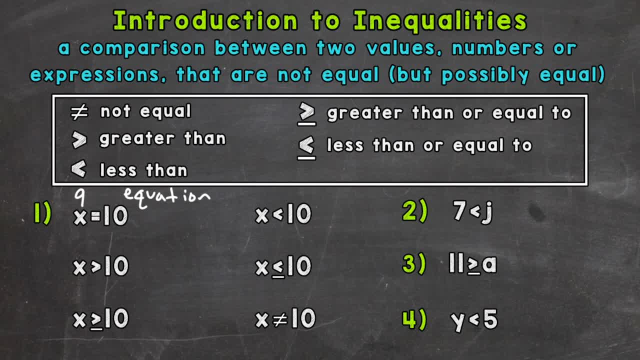 So x is greater than 10 here. So any number greater than 10 is greater than 10.. So any number greater than 10 is greater than 10.. So any number greater than 10 is greater than 10.. There's an infinite amount of correct solutions. 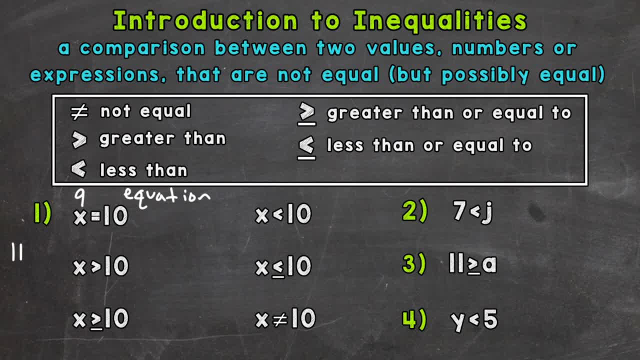 So, for example, 11 would work, 50 would work Or 150.. It doesn't matter Anything. greater than 10 would be a solution for x, for that inequality. Now, 10 would not be a solution because x has to be greater than 10.. 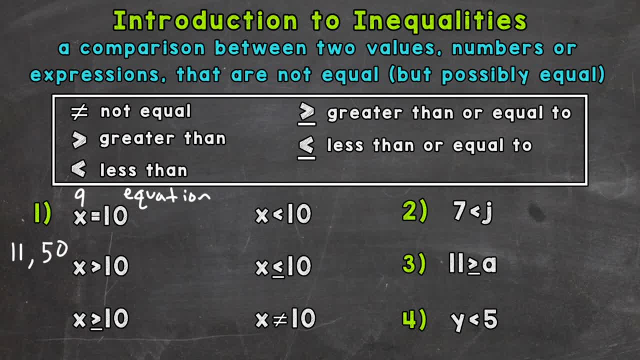 Is 10 greater than 10? No. Now the third inequality down right here is: X is greater than or equal to 10.. So all of those solutions we talked about, for X is greater than 10,, 11,, 50,, 150,. 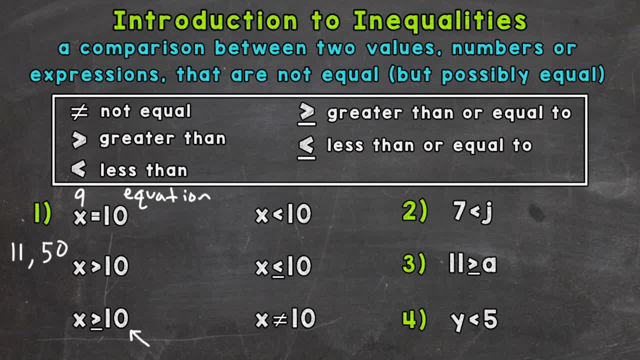 anything greater than 10 would be a correct solution, just like the one above, But this one, 10, is a correct solution as well. So 10 would work for this, because 10 is greater than or equal to 10.. So when we talked about the possibility of the values being equal, 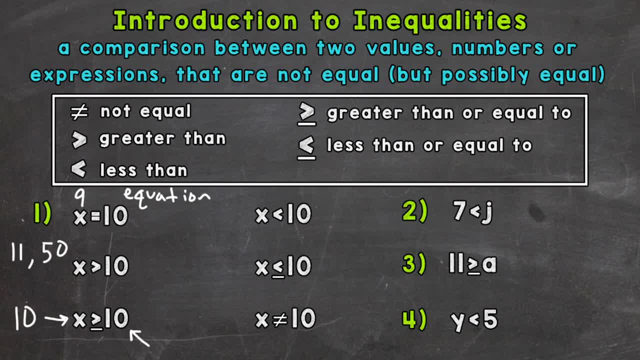 when we have that or equal to, we can have an equal solution there to the given value. So just to recap these two inequalities right here, any number greater than 10, 10 would be a correct solution, But they differ because the bottom one here. 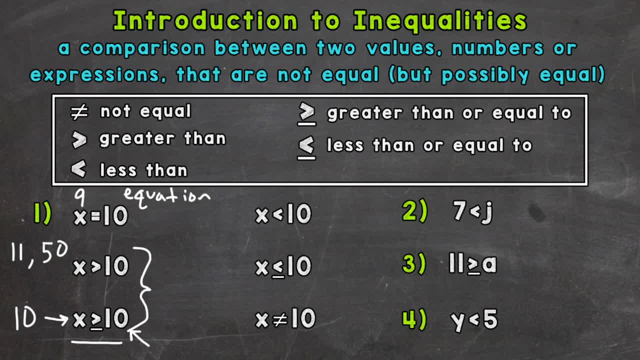 10 is included in the correct solutions because we have X is greater than or equal to 10.. So let's move on to this inequality right here, where we have X is less than 10.. So any value less than 10 would be a correct solution. 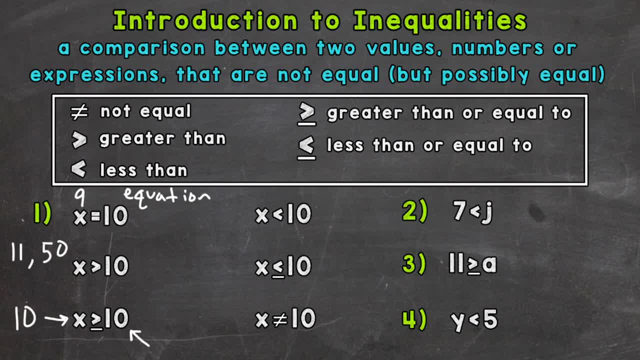 when we have that or equal to, we can have an equal solution there to the given value. So just to recap these two inequalities right here, any number greater than 10, 10 would be a correct solution, But they differ because the bottom one here. 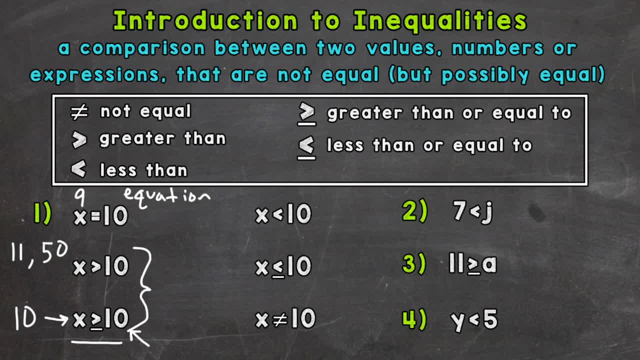 10 is included in the correct solutions because we have X is greater than or equal to 10.. So let's move on to this inequality right here, where we have X is less than 10.. So any value less than 10 would be a correct solution. 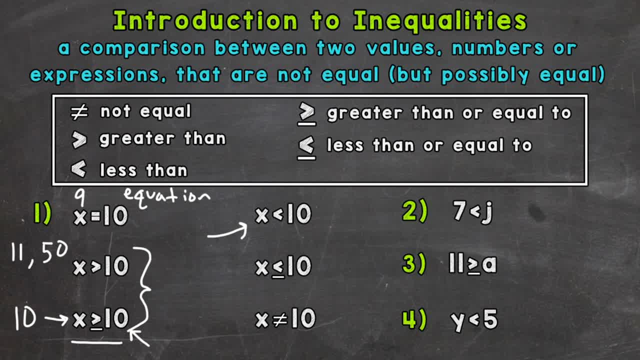 So 1,, 2,, 8, negative 8.. Whatever the case may be, Again, we have infinite solutions to that inequality. Now, 10 would not be a correct solution. 10 is not less than 10.. But for this inequality here we have, X is less than or equal to 10.. 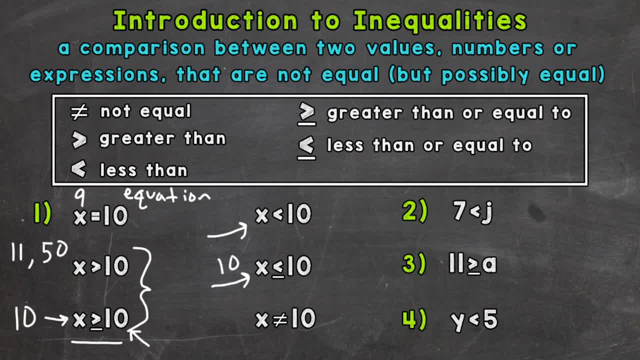 So 10 would work for this one, but not the top one. So you can see the difference between the less than sign and X is less than 10.. And then the X is less than or equal to 10.. So again, these two inequalities right here. 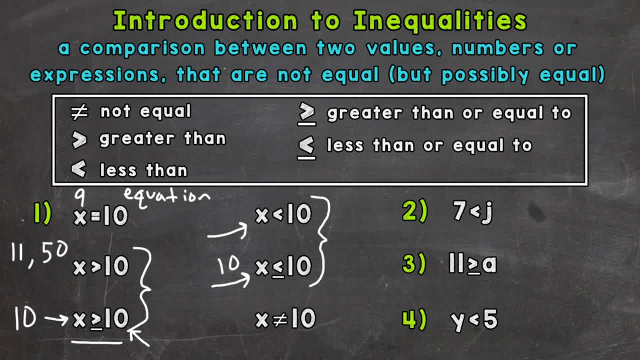 any value less than 10 would be a solution. but the less than or equal to, we can include 10 in those solutions. And then, lastly, we have: X is not equal to 10.. So value that's not 10 would be correct there. So 8,, 9, negative 20,, whatever the case may be. 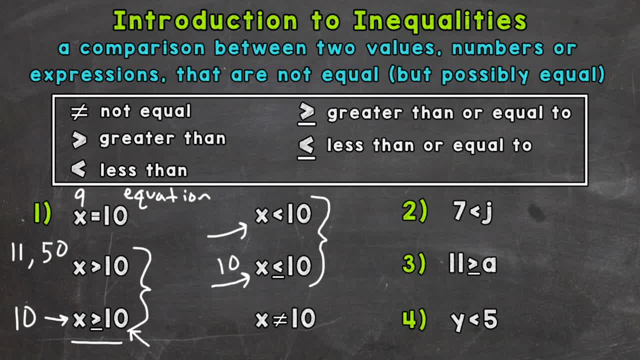 the only incorrect solution would be if we were to put 10 in there. Is 10 not equal to 10?? No, that doesn't make sense. So any value other than 10 would work for that last inequality. So let's jump over to numbers 2, 3, and 4 and come up with some correct solutions to those. 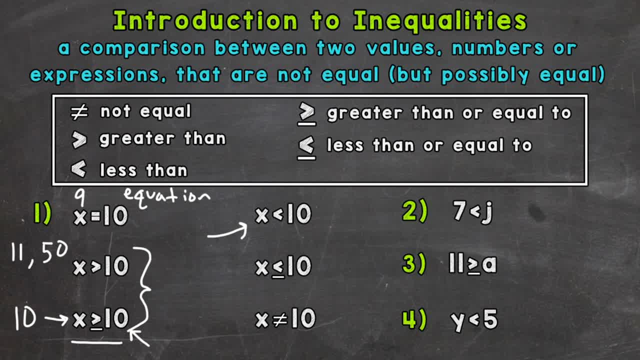 So 1,, 2,, 8, negative 8.. Whatever the case may be, Again, we have infinite solutions to that inequality. Now, 10 would not be a correct solution. 10 is not less than 10.. But for this inequality here we have, X is less than or equal to 10.. 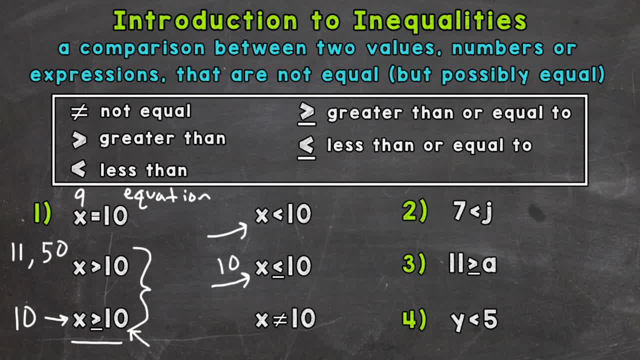 So 10 would work for this one, but not the top one. So you can see the difference between the less than sign X is less than 10, and then the X is less than or equal to 10.. So again, these two inequalities right here. 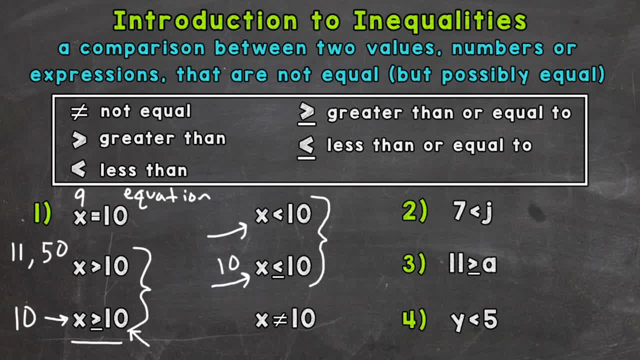 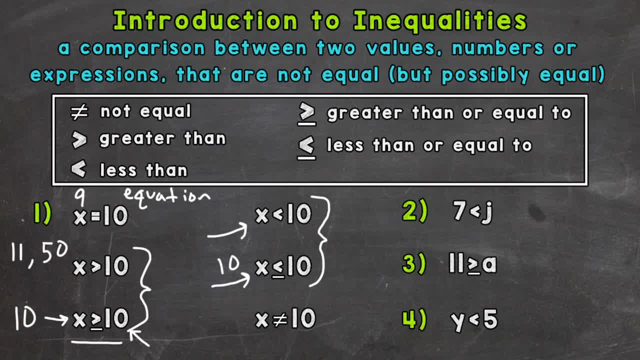 Any value that's not 10 would be correct there. So 8, 9, negative 20,. whatever the case may be, the only incorrect solution would be if we were to put 10 in there. Is 10 not equal to 10?? No, that doesn't make sense. 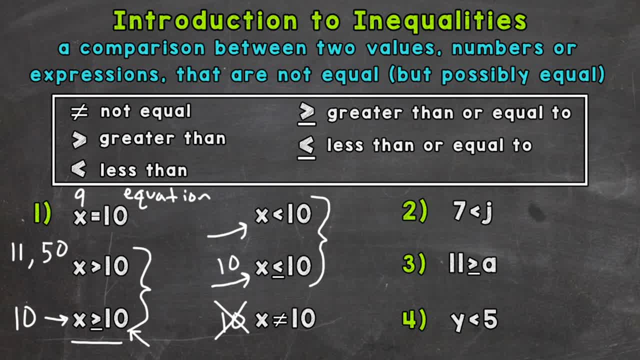 So any value other than 10 would work for that last inequality. So let's jump over to numbers 2,, 3, and 4 and come up with some correct solutions to those inequalities. So number 2, we have, 7, is less than j. 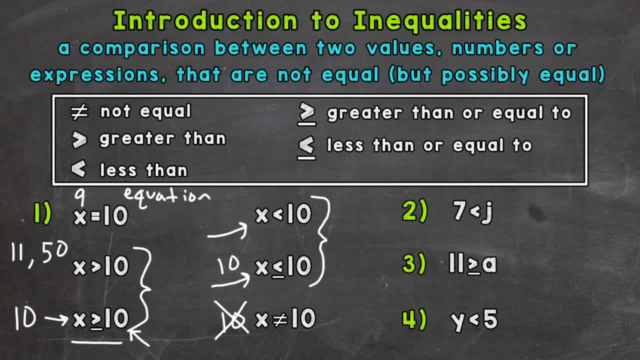 So any value greater than 7 there, because j, that side, has to be greater than 7.. So anything greater than 7 would work. So we could do 8.. Ah, 52 or 100.. Again, an infinite amount of solutions there.